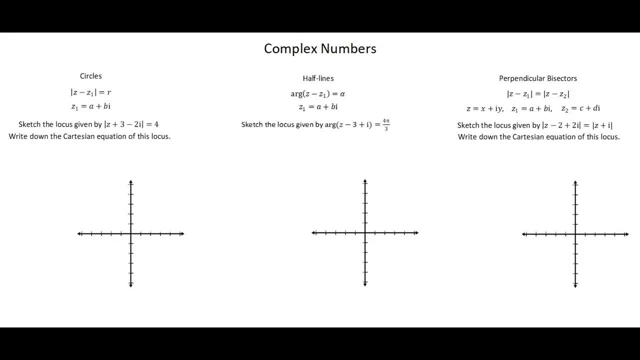 Hi, I'm Thomas, Welcome back. Our topic is complex numbers. In this lesson we'll learn how to draw a locus of points in an Argan diagram to represent complex numbers, Starting with circles. the general form for a circle is the modulus of z minus z1 equals r. z1 equals a plus bi. 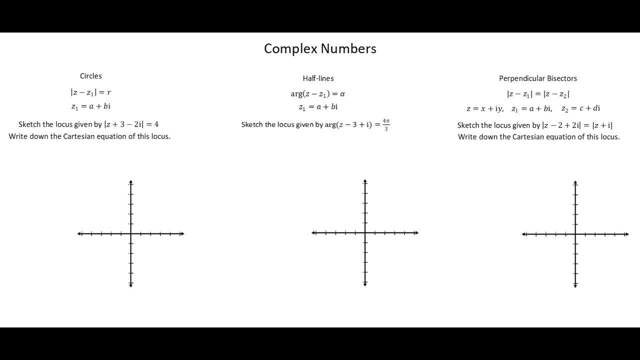 Our requirement reads: sketch: the locus given by the modulus of z plus 3 minus 2i equals 4.. Write down the Cartesian equation of this locus. I'll begin by rewriting the equation to clearly identify z1, the modulus of z minus brackets, minus 3 plus 2i. 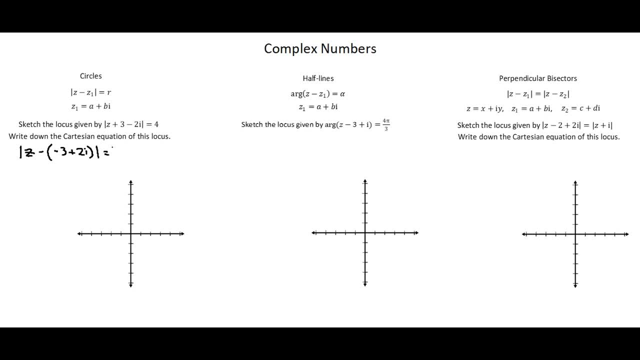 Close brackets. Modulus sign equals 4.. Now I have identified the z1.. Our general equation, z minus z1, is now z minus quantity negative, 3 plus 2i. The significance of z1 is that it provides the coordinates of the center. 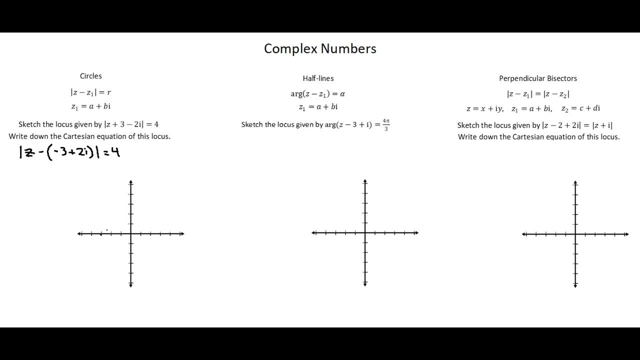 So negative 3 plus 2i will be at negative 3, positive 2. r, the right side of the equation, is the right: The radius of the circle. So we have a circle with the center at negative 3, 2, a radius of 4.. 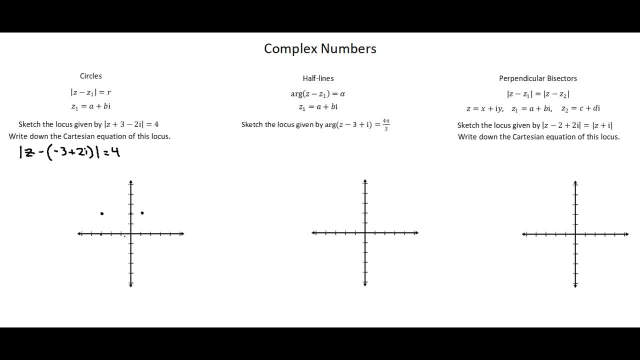 So our circle will extend to the right to the point 1, 2.. We'll extend to the left to the point negative 7, 2.. We'll extend up and we'll extend down. When we connect these points, they form a circle. 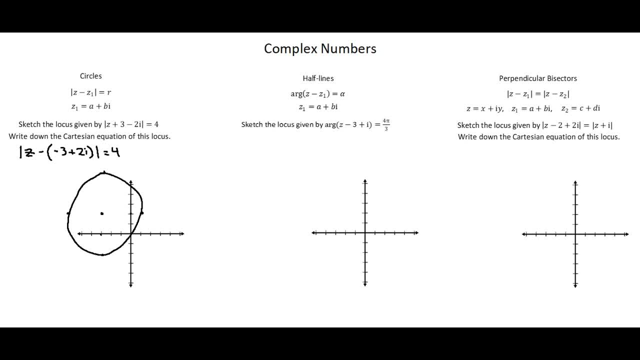 And this is the locus represented by the equation. given The second requirement, Write down the Cartesian equation of this locus. The Cartesian equation of a circle with center negative 3, 2 and radius of 4 is x plus 3 squared plus y minus 2 squared equals the square of 4, which is 16.. 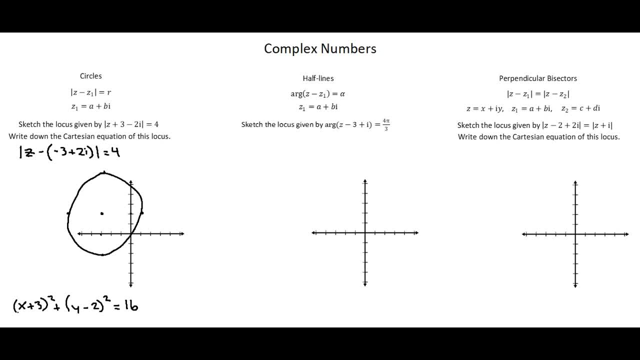 Next half lines: The general equation Argument of z minus z1 equals Alpha, z1 is a plus bi. Our requirement Sketch the locus given by argument z minus 3 plus i equals 4pi over 3.. Again, I want to manipulate my equation to clearly identify z1. 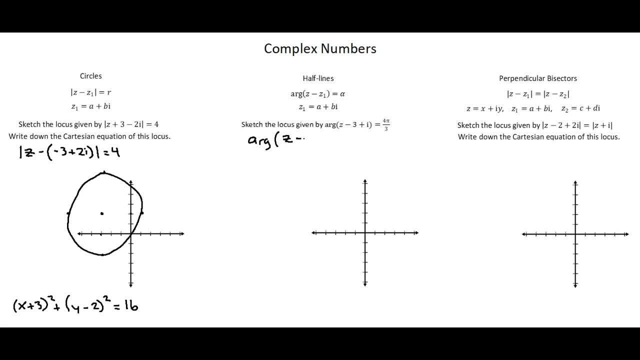 So I will write argument of z minus quantity 3 minus i equals 4pi For a half line. the significance of z1 is that it represents our starting point. We want the coordinates 3 and negative i. From here we're going to extend at an angle of 4pi over 3, working our way counterclockwise from a horizontal extension from our starting point. 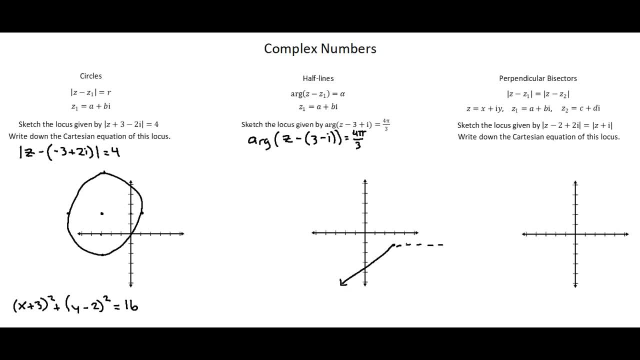 4pi over 3. going down and to the left, Counterclockwise, from our starting position, This represents the half line of the equation. given This is a half line because it's extending infinitely in one direction: We start at 3 negative 1 and extend infinitely at an angle of 4pi over 3.. 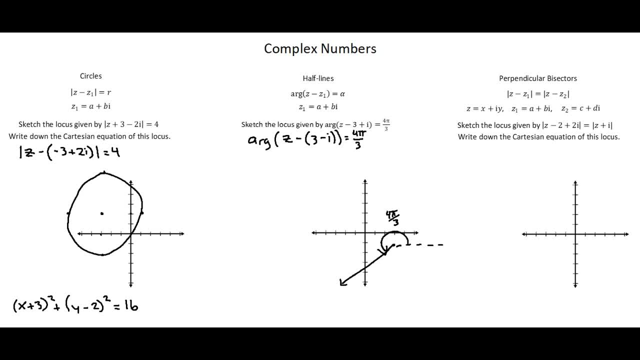 Now perpendicular bisectors. Our general equation: The modulus of z minus z1 equals the modulus of z minus z2.. Where z equals x plus iy, z1 equals a plus bi And z2 equals c plus di. Our requirement Sketch: the locus given by modulus z minus 2 plus 2i equals modulus z plus i. 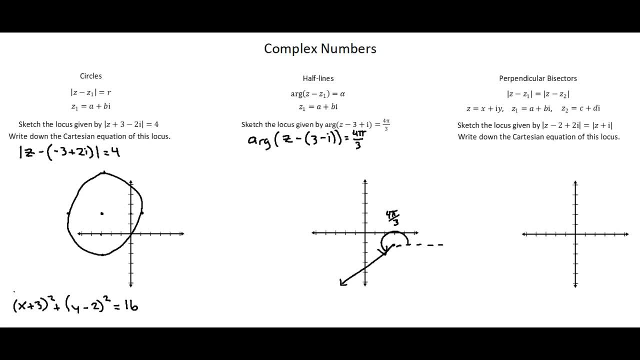 Write down the Cartesian equation of this locus. I want to clearly identify z1 and z2.. So I'll rewrite the equation as: modulus z minus quantity 2 minus 2i equals modulus z minus quantity, zero minus i. I've included that zero to show that the complex number doesn't have a real part. 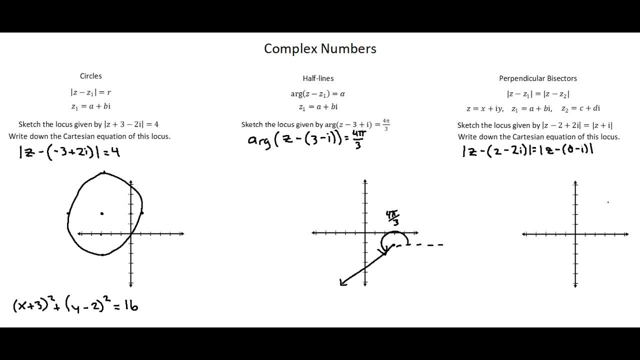 It's a purely imaginary number That will help us in identifying the correct coordinates in our argand diagram: z1 to minus 2i And z2, zero minus i. I now want to identify the perpendicular bisector, So I'll start by finding the midpoint. 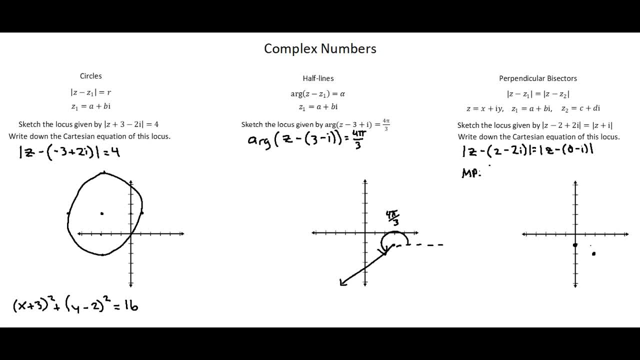 The midpoint is the x values added and divided by 2.. 2 plus 0 over 2. And the y values added and divided by 2.. Negative 2 minus 1 divided by 2. We end up with 1 negative 3 over 2.. 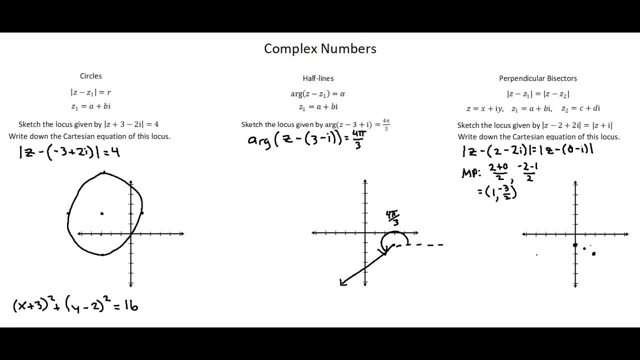 The perpendicular bisector requires the calculation of the gradient of the line segment connecting z1 and z2.. We can calculate our gradient as: m equals the difference in y values Negative 2 minus minus 1.. Over the difference in x values To minus 0. 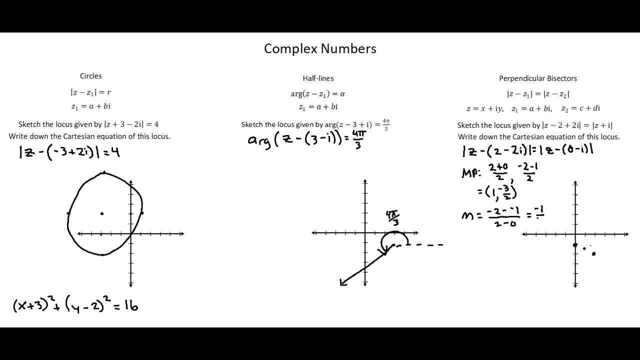 Which equates to negative 1 half. The perpendicular to that will be 1 over negative m, Which gives us a slope of positive 2.. And now I can draw in my perpendicular bisector. I'll also, with a dotted line, connect. 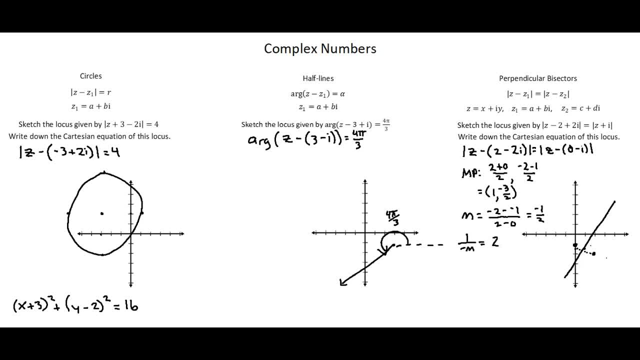 z1 and z2.. This is the locus of points represented in the given equation. Now, before we go to part 2 of the perpendicular bisectors example, as an enhancement to each of these three examples, I'm going to go back to the Argand diagram. 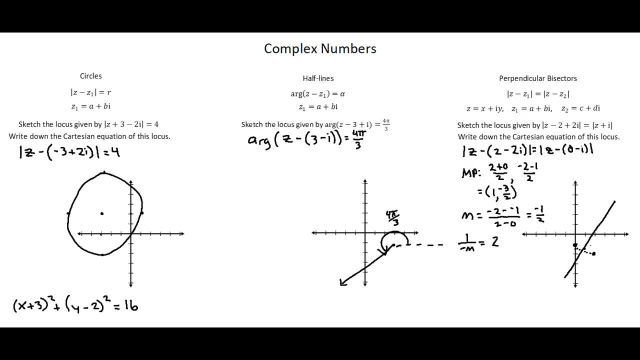 I'll label the axes and label the z1s And, in the case of our third example, the z2.. Now, looking back at our circles example, I've labeled the center as negative 3 plus 2.. And negative 3 plus 2i. 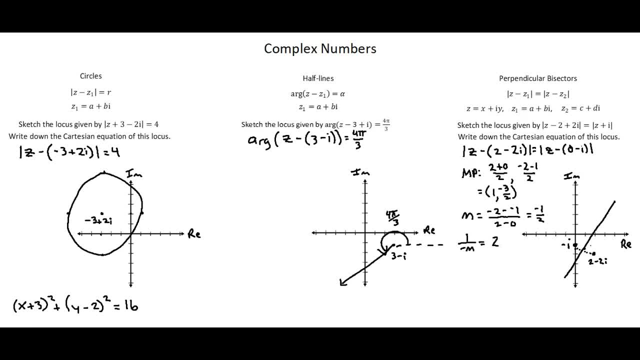 In the half lines example, I've labeled this starting point as 3 minus i And in the perpendicular bisector example, I've labeled z1 as 2 minus 2i And z2 as negative i. And now, returning to the perpendicular bisectors example,